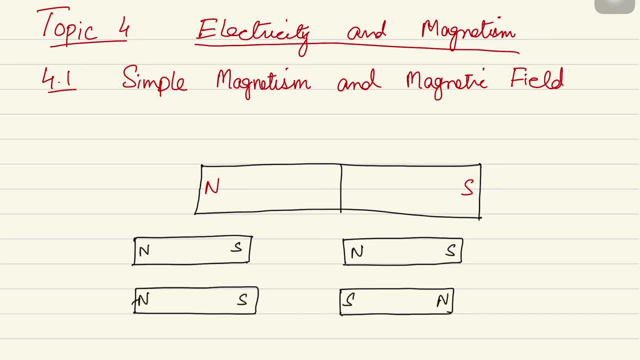 that's north pole, that's the south pole, that's the south pole and this is the north pole. now you see, in this figure we have the same poles like poles in front of each other. so these two magnets will be repelled. so in this case we will see the force of attraction between the 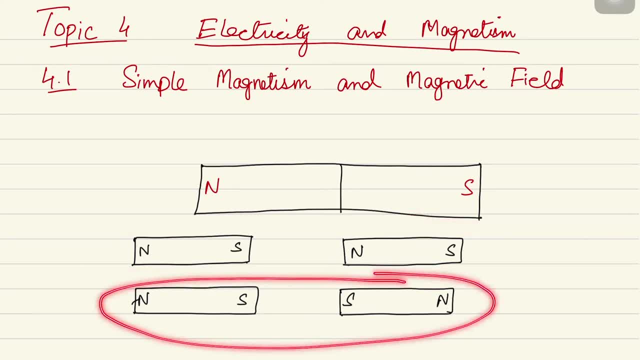 magnets, and in this case we will see repulsion among these magnets. so from here we can conclude that the like poles attract, like poles repel each other and the unlike poles attract each other. so that's the main phenomena of the magnetism. i'll write it here. 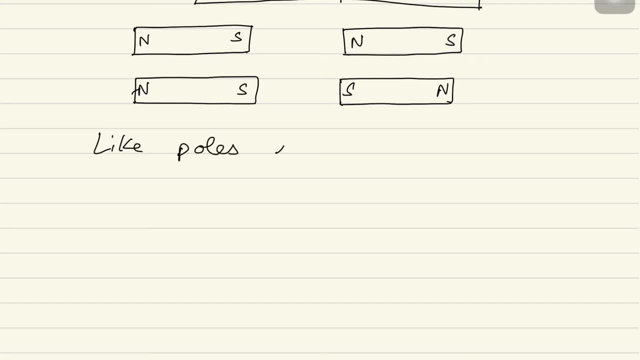 like poles repel each other and the unlike poles attract each other. so these are the two basic points that you have to remember about the magnets, that the like poles. they repel each other. for example, um north, north repulsion, south, south repulsion. but in the unlike poles, for example, north, south or south north, 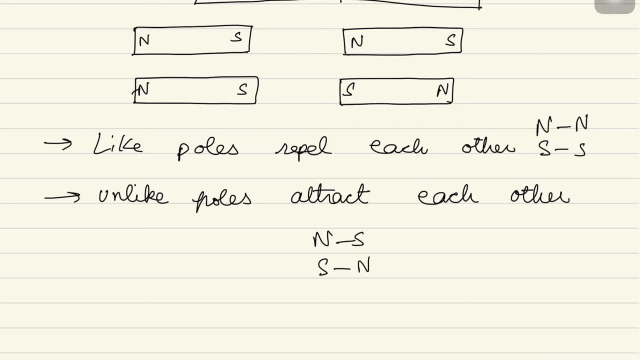 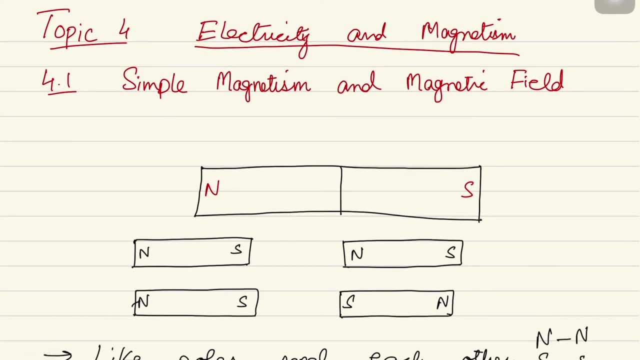 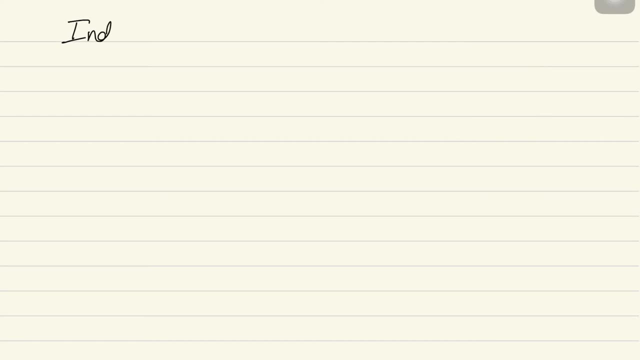 there will be attraction. so that's the basic phenomena of magnetism. now in the next discussion we'll discuss about the induced magnetism. what is induced magnetism? so induced magnetism, induced magnetism is basically. it's a phenomena where we pass current through through a magnetic material and it converts into a magnet. 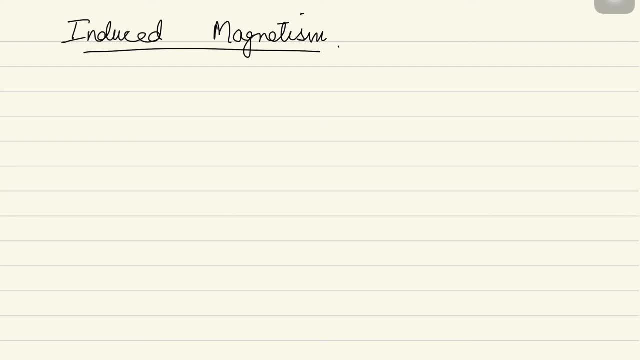 for example. let's take an example over here. let's suppose, um, there's a coil. or before that, let's take a steel rod over here, that's a steel rod. okay, we wrap a coil around that steel rod like this: that's the coil. and over here we'll attach this coil with a battery. 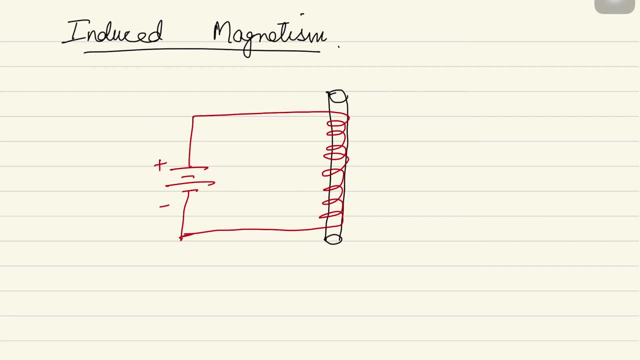 that's the positive terminal, that's the negative terminal. so here the current will flow through this coil and in the meanwhile this iron piece will become a magnet. so that is the phenomena of induced magnetism. when we pass the current through this coil there will be a magnetic field. temporary magnetic field will be generated in. 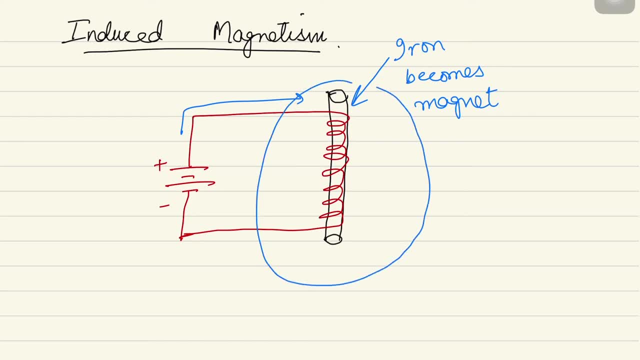 and, as a result of that, this iron material will become a magnet. so that's the phenomena of induced magnetism, where magnetism, magnetic field, is produced by the current getting through a conductor, and we will discuss that in detail as well. all right now. the next thing that we have to discuss is the difference between the magnetic 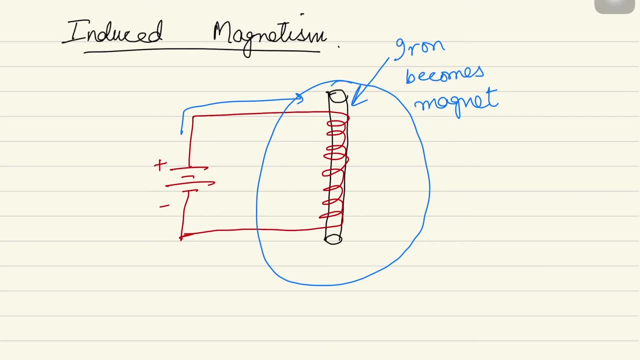 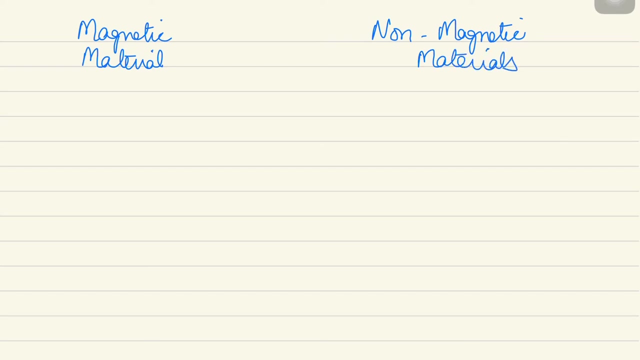 and the non-magnetic material set is quite simple and easy to understand. so magnetic and non-magnetic materials, non-magnetic materials. so the magnetic materials are the ones that are attracted towards the magnet and the non-magnetic materials are the ones that are not attracted towards the magnet. it's that much simple. 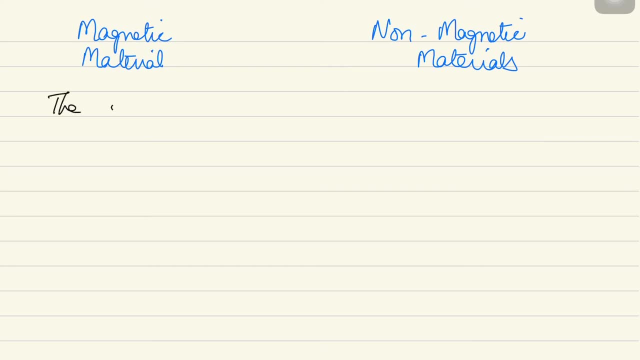 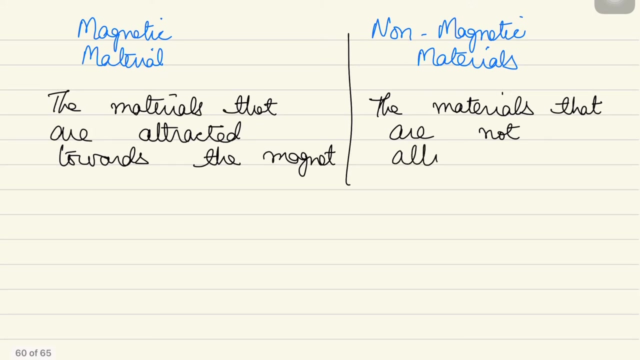 so i'll write it over here: the materials that are attracted towards the magnet. these are the magnetic materials, and the non-magnetic materials are the ones, the materials that are not attracted towards the magnet. so these are the non-magnetic materials. it's that simple. for example, 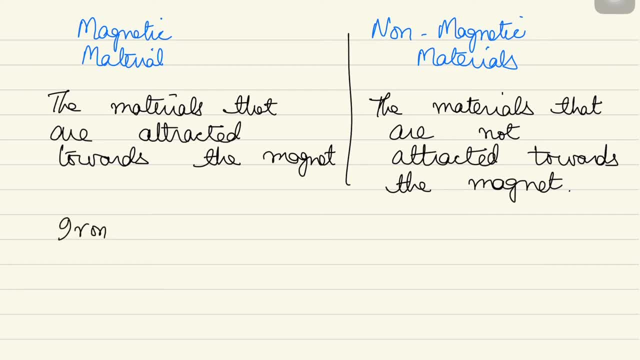 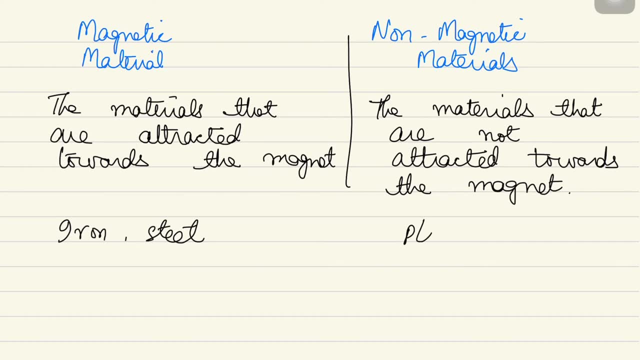 in magnetic material, you can take the example of iron, you can take the example of steel, up to some extent, but in non-magnetic materials, you can take the example of plastics, wood and the materials like that. that right, so yeah, these are the differences between the magnetic and the non-magnetic. 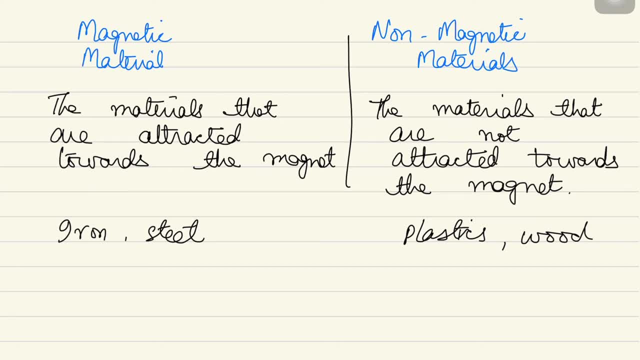 materials. now we have to discuss about the properties of some. we have to discuss the difference between the properties of the temporary magnets and the permanent magnets. so, um, i discussed the example of that current coil, like current passing through a coil, and that iron piece became a temporary, a magnet. so that was the temporary magnet and the magnet and the 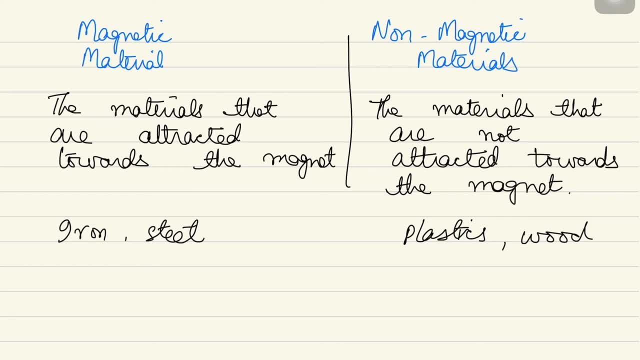 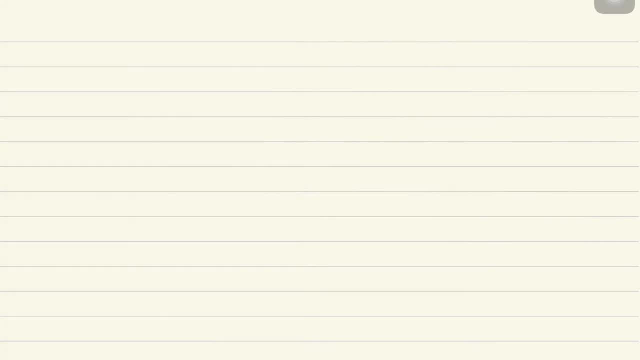 magnets that are made up of steel. they are the permanent magnet. okay, so let me just discuss it again: temporary magnets and the permanent magnets. temporary magnets and the temporary magnets. permanent magnets, temporary magnets, are the ones that that magnetized for some time and then they become normal, but the permanent magnets are the ones. so once you magnetize them after some time, they'll. 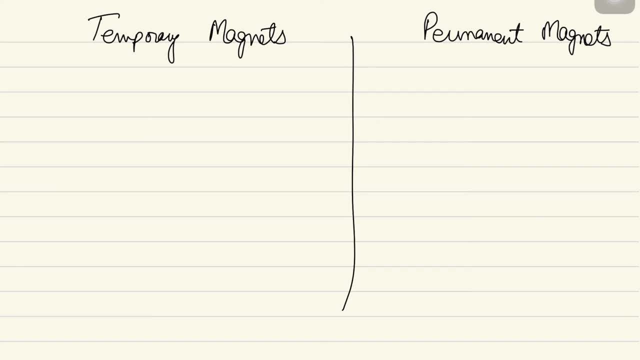 become fully magnetized and then they will not be demagnetized. so those are the permanent magnets. in temporary magnets we are, we consider the magnets consist of of a iron. in permanent magnets we just we take the magnets that are made up of steel, for example. this is the iron piece, like the same example as i discussed before. that's iron piece. 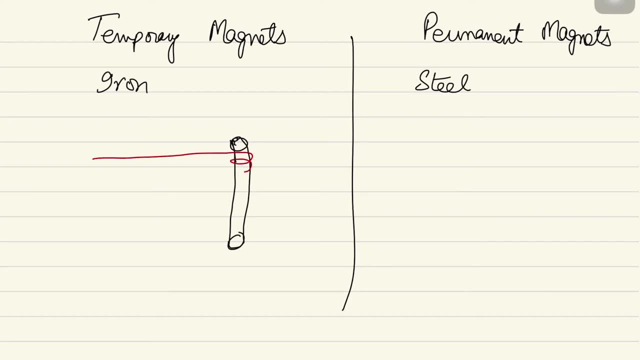 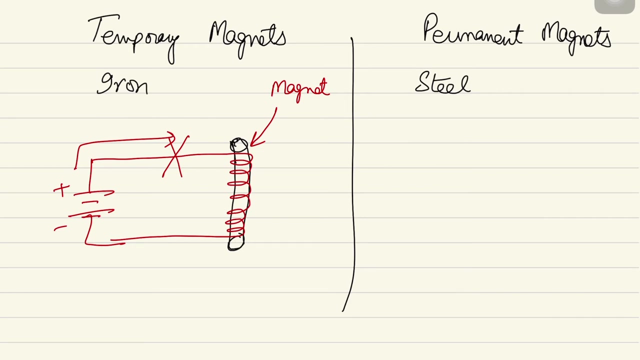 and we wrap a wire around it. so it becomes a coil and from that coil we pass the electricity. if we pass the electricity to that coil and this iron piece becomes a magnet, if we switch off this electricity, then this iron piece will become, will be no more a. 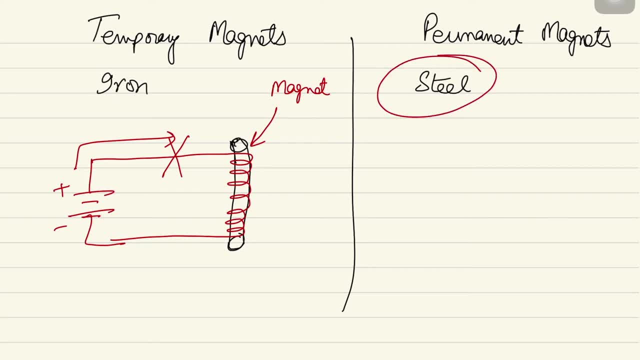 magnet. but in case of steel, if you do the same in case of steel, it will be permanently magnetized. once it is magnetized it is, and we turn off the current, it will not be demagnetized. so such magnets are the permanent magnets and other ones are the temporary magnets. all 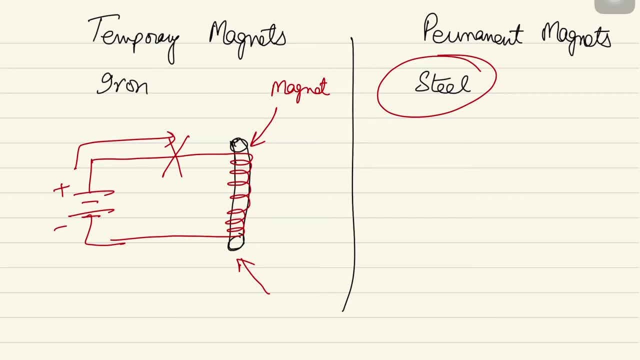 right. so yeah, that's the difference between the permanent and the temporary magnets. now we will discuss about the magnetic field. like, what is the magnetic field? so magnetic field? so magnetic field is nothing but a region where a material experiences a magnetic force. okay, i'll write it over here: the region or space. 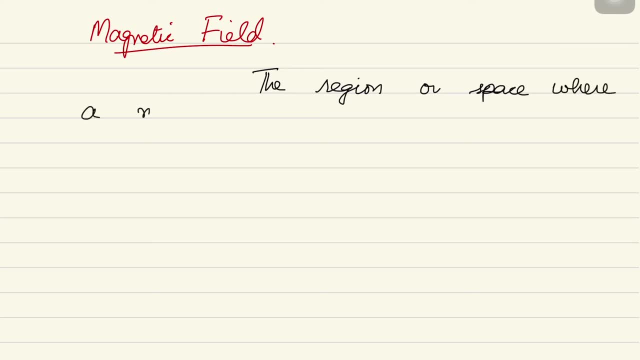 where a magnetic material not a simple material, but a magnetic material, not non-magnetic, where a magnetic material experiences magnetic force, that region or space is called the magnetic field, for example. um, let's put a bar magnet. let's suppose i put a bar magnet over here. 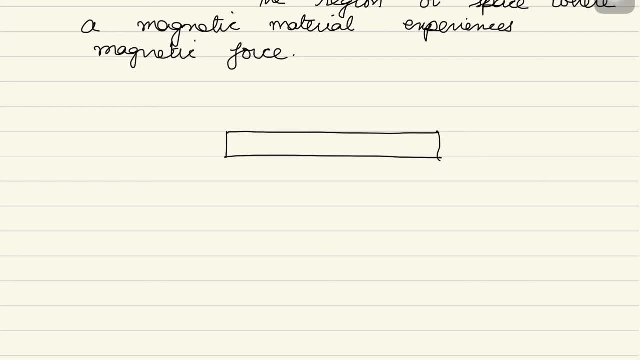 that's the north pole, this one is the south pole. now the magnetic magnetic field lines will start from the north pole and the magnetic field lines will start from the north pole and they will end at the south pole. magnetic field lines are basically there to represent the magnetic field, to represent that region, so they will start from the north pole. 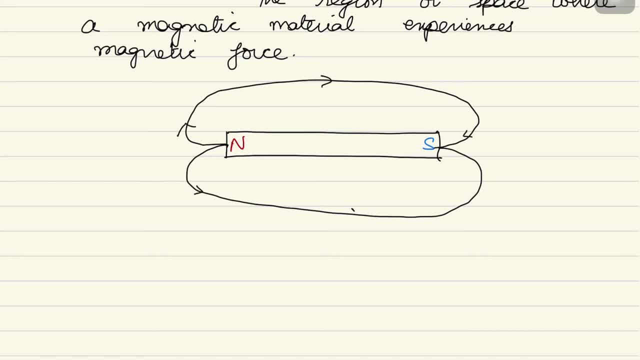 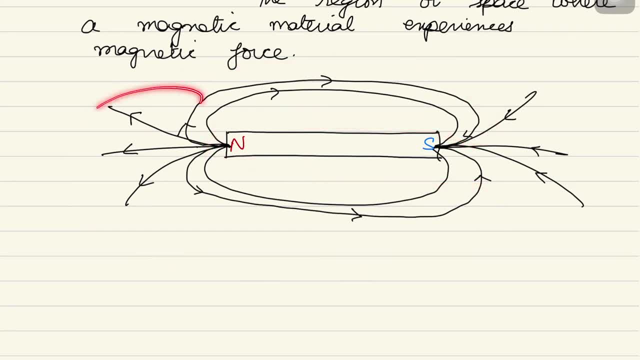 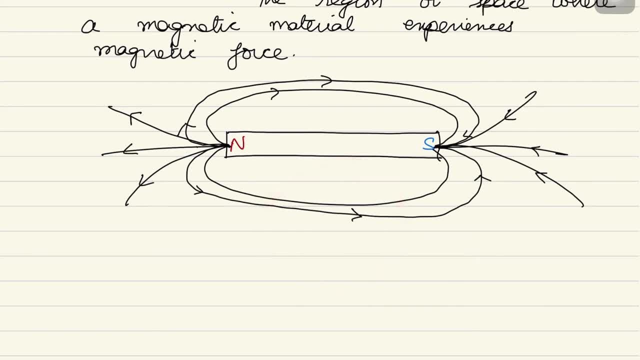 but, like in the region over here, the magnetic materials will experience less magnetic force. again, in this region, the magnetic materials will experience strong magnetic force. so that's how it works. so that's how we explain the magnetic field and that's how we represent the magnetic field. um, with the magnetic field lines, they start off from the 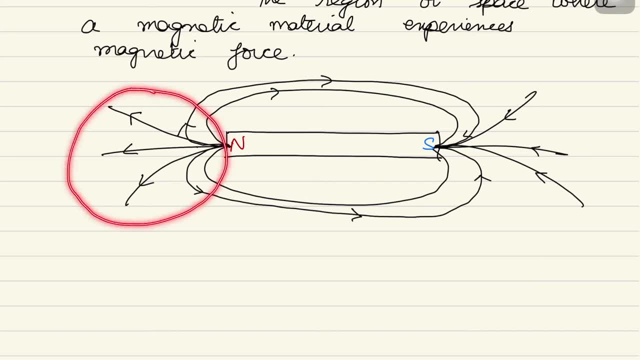 north pole. that's why the arrows are away from the north pole. they move towards the south pole. so that's why the arrows are towards the south pole. that's the thing that that you have to remember. okay, now let's suppose, if you put, if you place the iron, small pieces of iron, around this bar magnet. 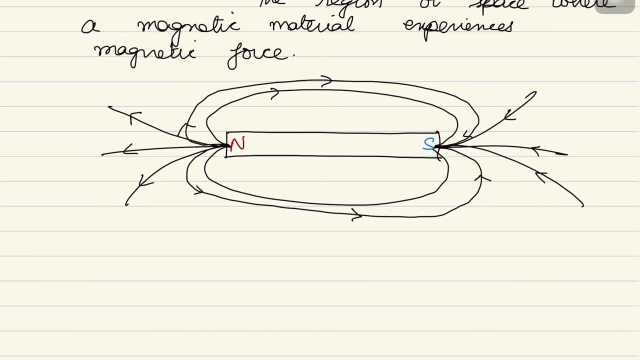 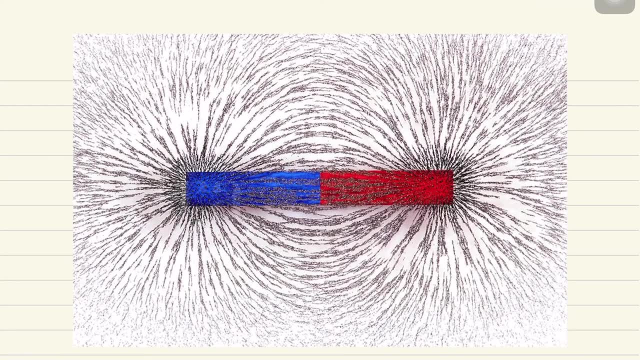 we will see a pattern of the magnetic field lines, so i'll show you a picture over here. there you go. so look at this: this is the north pole and that's the south pole, or you can think of this as the north pole and this as the south pole. now look at this. these are the iron fillings. 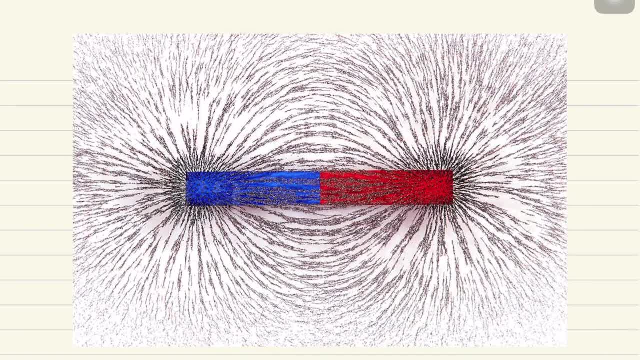 like small pieces of iron. we have just distributed these small pieces of iron and look at that, they have formed a pattern. you see, here you go. that's a pattern that has been formed. now this pattern is showing the magnetic field around this bar magnet. now let's discuss different areas one by one. for example, 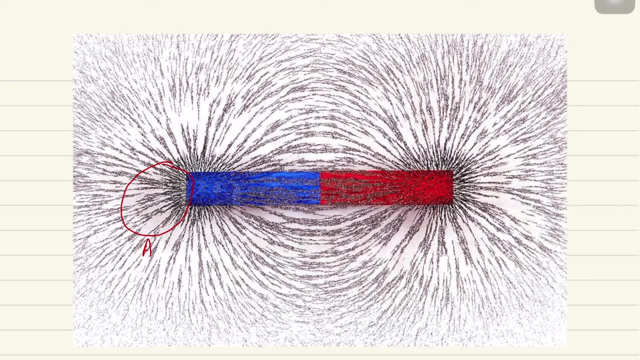 area number a, area number b and area number c. now, as you this, as you see, area number a, the iron fillings are pretty much close to each other. since the iron fillings are pretty much close to each other, so we can say that they have. since they are close to each other, it means it has strong magnetic field in region a. 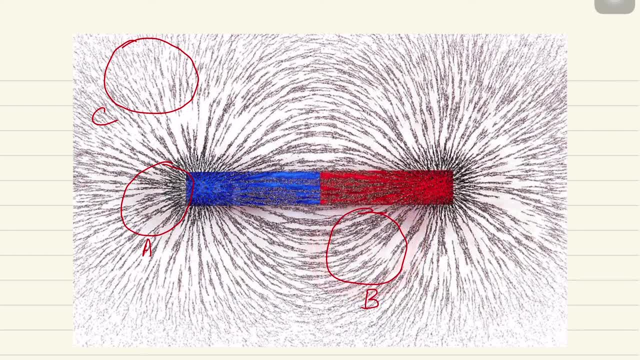 in region b the iron fillings are at the moderate distances from each other. so since they are at the moderate distances from each other, we can say the magnetic field line is, the strength of the magnetic field is like moderate. but in region c the iron fillings are pretty much away from each other. so we can say that 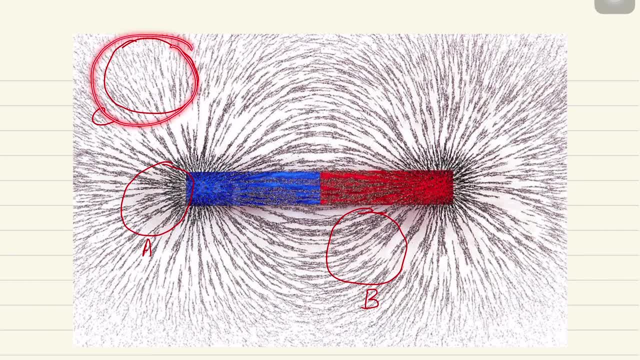 the magnetic field is weak in region c. so it all depends on these iron fillings. if they are close to each other, we'll say the magnetic field is strong. if they are away from each other, we'll say the magnetic field is weak. so that's how we represent the magnetic field, by 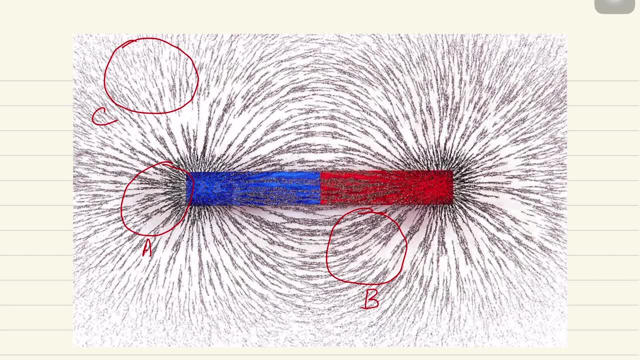 using um, these iron fillings. and these iron fillings are basically, they're making a pattern of the magnetic field lines, and where the lines are close to each other, we'll say that's the region of strong magnetic field. and where the where those lines- magnetic field lines- are away from each other, we'll say that that is the region. 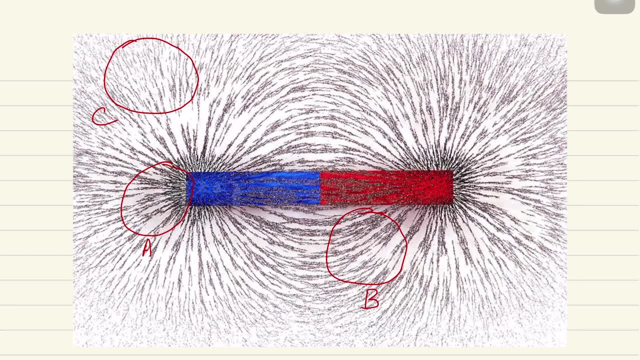 of weak magnetic field. and as far as the direction is concerned, the direction of the magnetic field lines are always from the north pole towards the south pole. so this is it about the bar magnet, about their poles- north pole, south pole- about the magnetic field, about the magnetic. 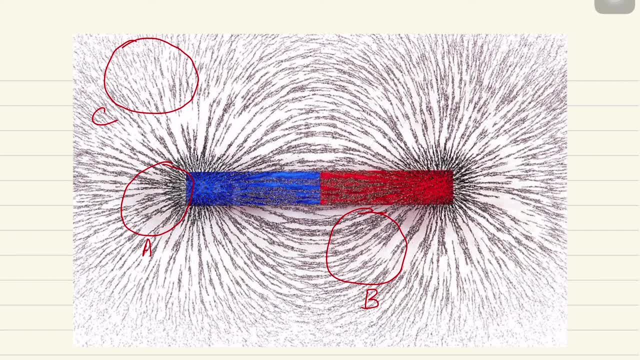 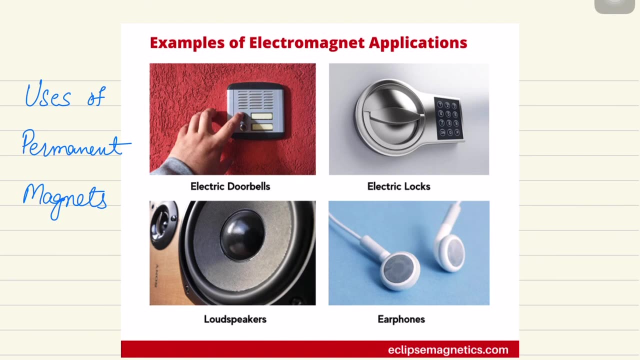 field lines their direction. it's all done. now the last thing of this topic that we have to discuss is the use of the permanent magnets and the electromagnets. so let's discuss the uses of the permanent magnets first, and then we'll discuss about the electromagnets. electromagnets are: 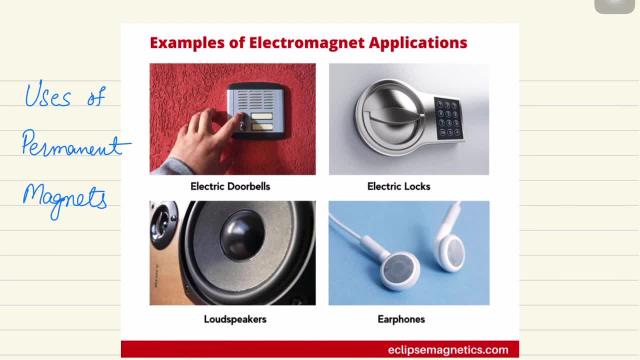 usually the temporary magnets. we categorize them, uh, in the temporary magnet, permanent magnets, they, they stay magnet all like till like, like throughout. but the electromagnets, or the temporary magnets, they stay magnet as like. they stay magnet until the current is passing through them. if the current stops passing through them, they become demagnetized. so 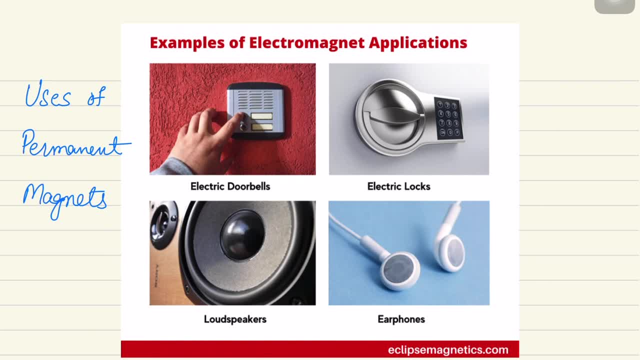 let's discuss the uses of some of the permanent magnets. number one: the permanent magnets they are like used in the electric door bills, in electric clocks, in loudspeakers and in the earphones. earphones and loudspeakers are categorized, i mean, in the same category, because loudspeaker are just the bigger version of the earphones. 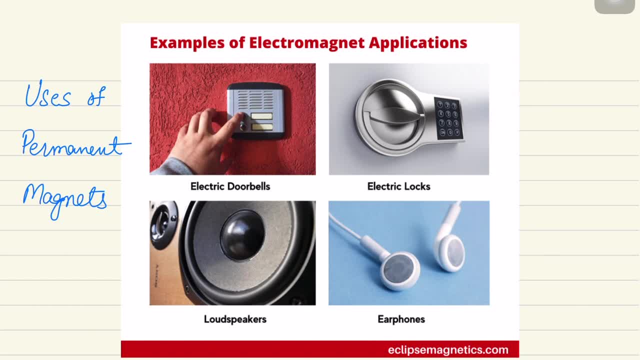 and electric clocks. they're used, electric clocks they're used in the electric doorbells. so these are the some of the main examples of the of the permanent magnets. okay, over here there it's written examples of electromagnet, electromagnet, electromagnet, applica. but in the loudspeaker we use permanent magnets, in the earphones we use the permanent magnets. 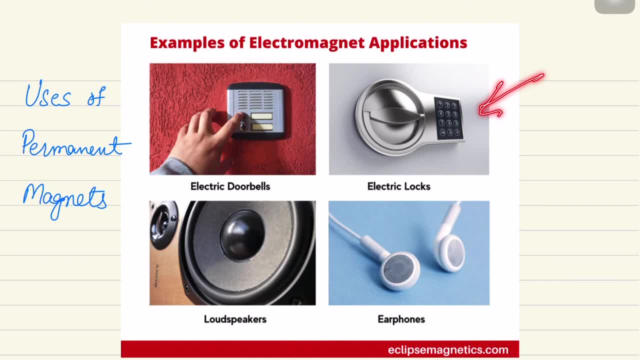 in the electric clocks up. to some extent we use permanent magnets, but usually we use the electromagnets. so you can say that these two are the examples of the permanent magnets and these two are the examples of the temporary or electromagnets, temporary magnets. or you can say: 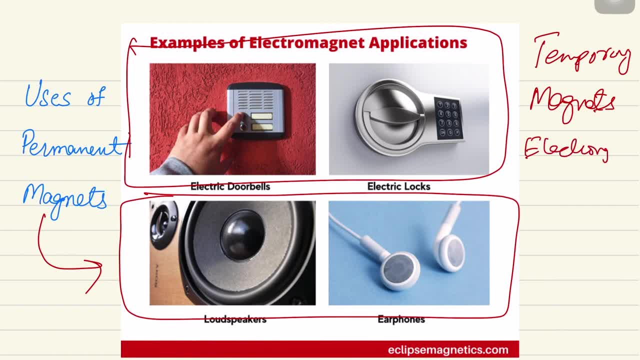 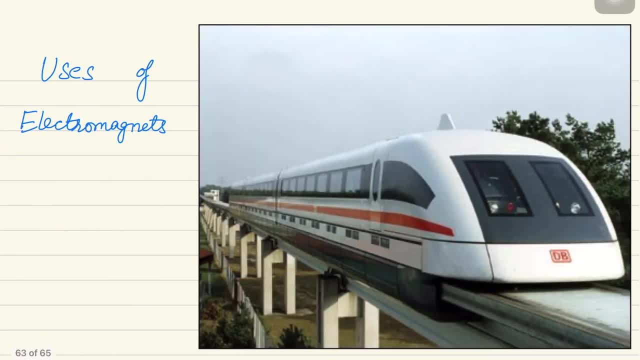 electromagnets. so you can say that these two are the examples of the permanent magnets. have some more examples of electro electromagnets, so let's discuss them. here you go. electromagnets: they are used in the magnetic levitation trains. so these strains, basically they use the concept of electromagn, they use the concept of 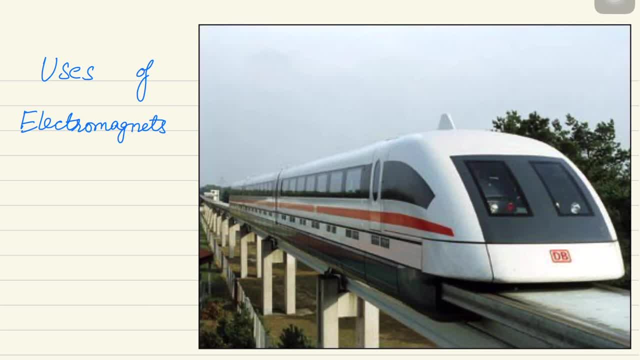 like poles repelling each other. so ideally it should stay in in air. so basically, this train does not touch the rail railway line, it just floats on onto the railway line. so that's why it's a very high speed electric train. now here's another example. this is the example of the. 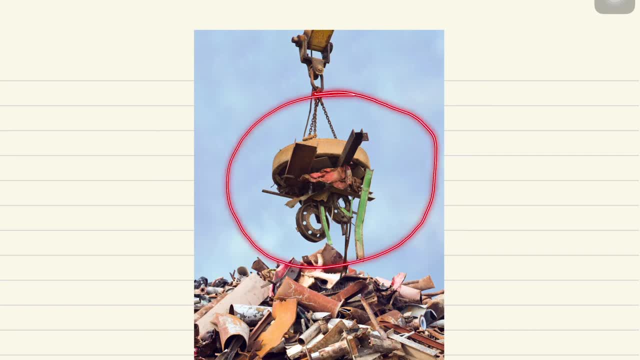 electromagnets. so this is the huge electromagnet that is used to lift the heavy weight, heavy metals. we also use such type of electromagnets in order to separate the iron pieces from the non-iron pieces, or from the magnetic materials from the non-magnetic materials. so this object. 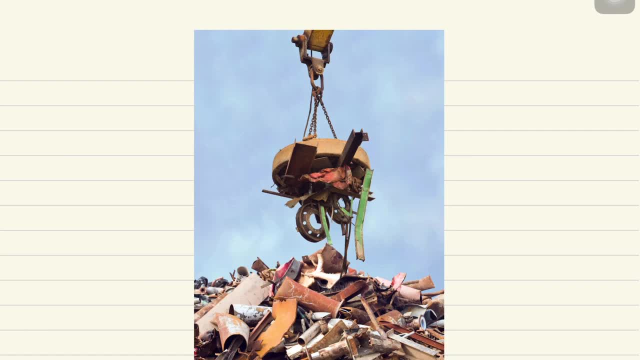 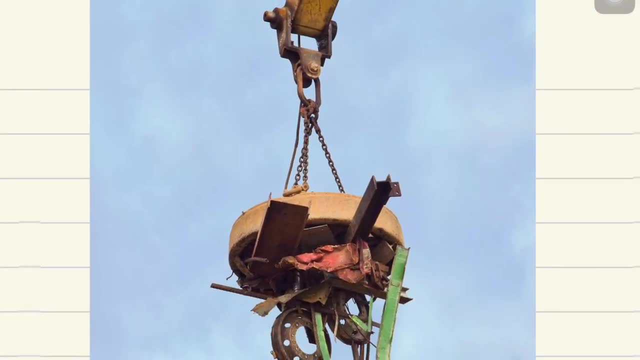 over here that you are seeing is an electromagnet. you see, over here, this is the wire. there you go. that's the wire, this is the wire. so the current is passing through this wire, which is turning it into an electromagnet, and this electromagnet is um pulling the heavy objects, the more current you 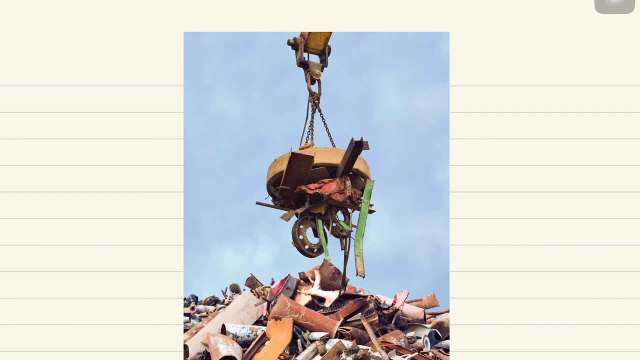 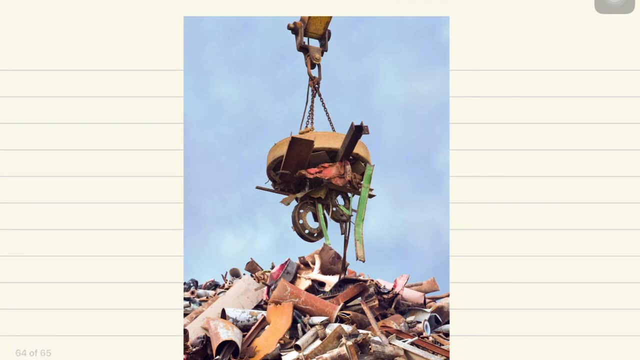 pass through the uh, through this iron structure, the more strong magnet it will it will be and the more heavy weight it will lift. okay, so these are some of the uses of the permanent magnets and the electromagnets. this topic was just simple: uh: basics of the magnetism and the magnetic fields. 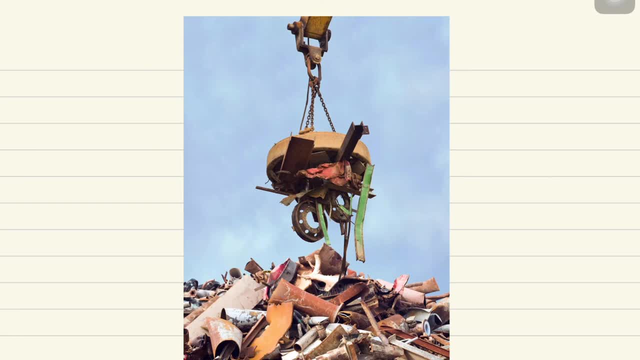 that you, that you should know. so we have discussed about the north pole, south pole- like poles repel, unlike poles attract, and about the bar magnet, about the magnetic field lines, the strength of the magnetic field and, at in the end, we have discussed about the uses of the permanent and